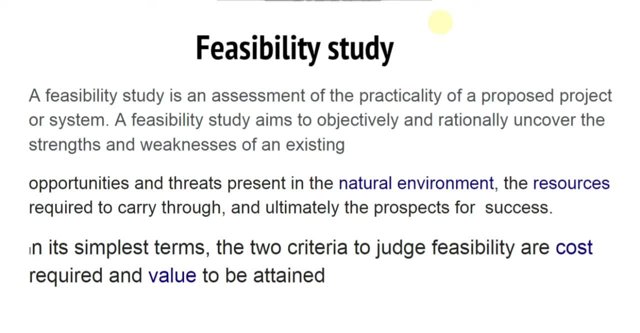 started if the feasibility report is not quite give the results. so we did not going towards to start the project. because a project will consume our time, cost and everything related to the resources. so feasibility study is the study of a project. whether the project is possible or not, whether the resource available resources. 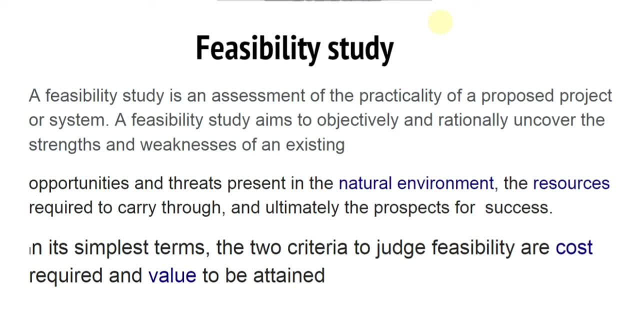 will support the project or not. so if the available resources, such as natural environment, impacts the cost, the time, the people efforts. so everything we study and we compare with the project that it is a support to the project or not. so the resources support to the project are not. so its general. 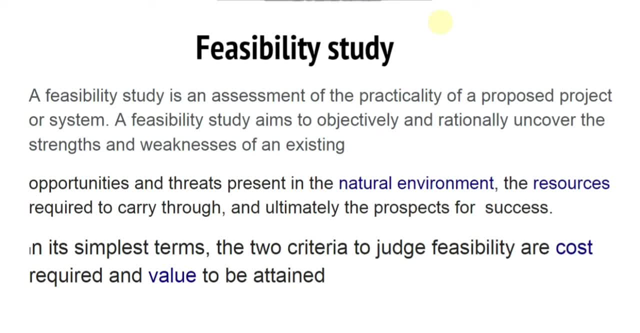 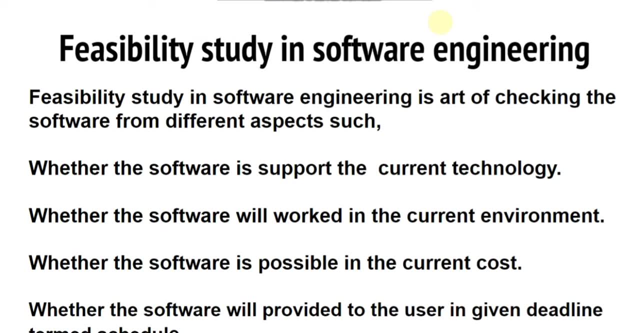 definition of feasibility study is the study of a project and whether the project is possible or not study. let's move towards feasibility study in software engineering. feasibility study in software engineering is the art of checking the software from different aspects, such as whether the, whether the software is support the current technology, whether the software will work in the current 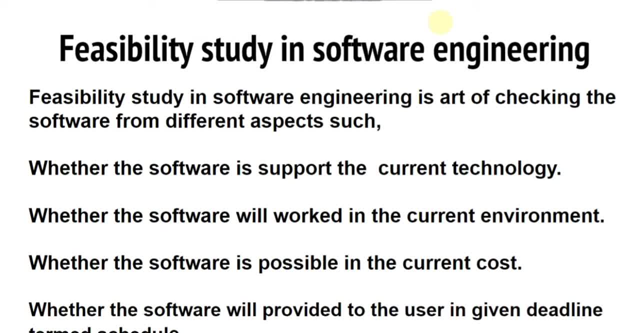 environment, whether the software is possible in the current cost or whether the software will provide to the user given deadline terms as schedule. so feasibility study is the study of our different aspects of project, such as the whether the software support the current technology or not. so if the software does not support the current technology or the hardware, 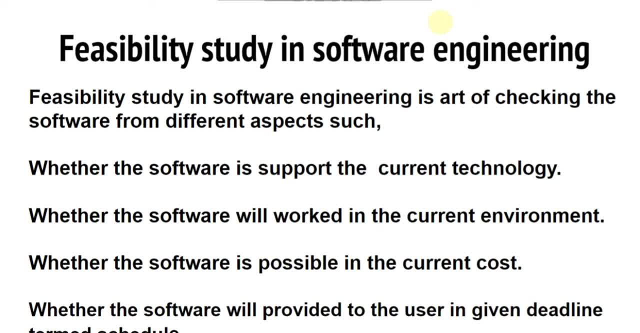 available, so it's useless. because when we start the project we invest a lot of thing: money, time, people, effort. so if the software are, if the project is not supported by the current technology, so it is useless. because the organization has some available technology equipments. so we make the software that if it will support the current technology, 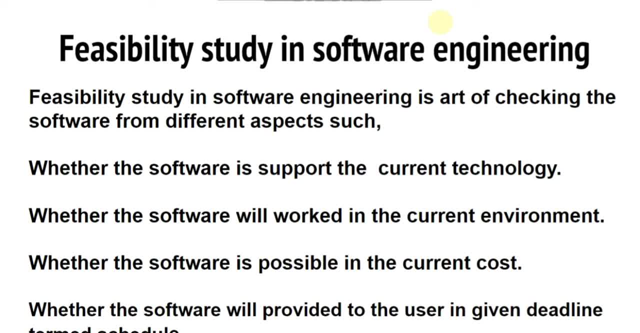 before going towards software development. so we will study the current technology available in the organization because if the are going to, if the software does not support the current technology, so it may lead a very huge cost to buy the technology, um Technology which is supported by the software. 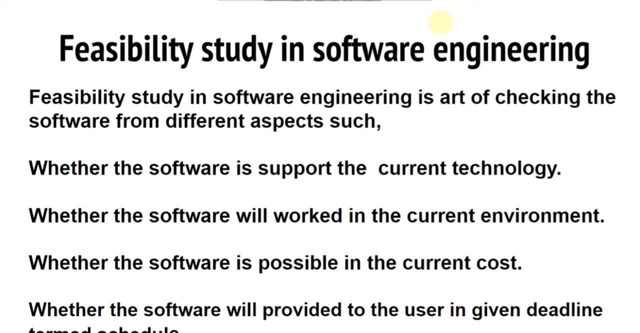 number. second point: whether the software will work in the In the current environment. so we study the environment, So if the software support the current environment or not. so we first study the environment. Environment contain a lot of things. so when the software Software will work in the current environment or not, is people are aware about the use of software? 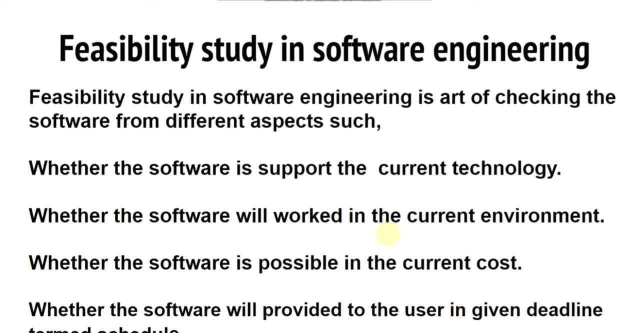 So it contain a lot of aspects. So whether the software is possible in the current cost or not. So when we estimate the cost, so if a project is completed or if a software is completed in $1,000, so we estimate out and whether the software will be completed in this cost or not, because 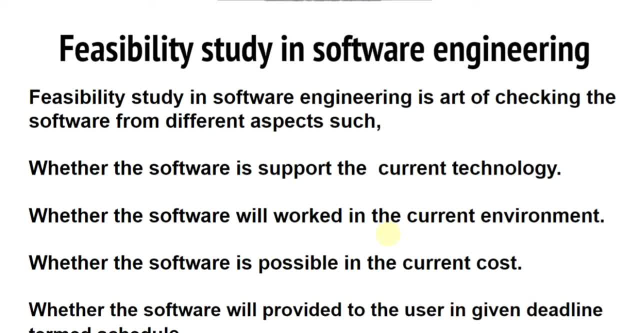 The software company will use the different resources such as time, money cost people, efforts, a lot of expenses, others. So that is why the feasibility study will study the cost estimate of the project, So whether the software will provide in the user given deadline term schedule. So with the help of feasibility study we schedule the software, whether the software will 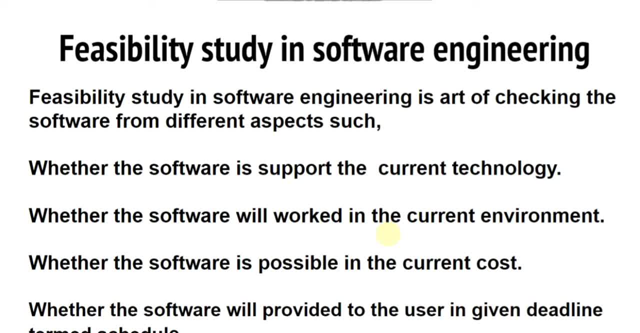 Will completed in the given time or not. the user want that. he want a software in two months. So the software. it is the responsibility of software company to study these things it whether it is possible or not In the given deadline. so it's all about the feasibility stream. So let's move towards a different types of feasibility. 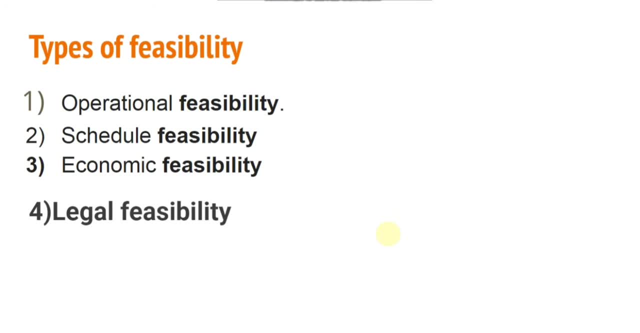 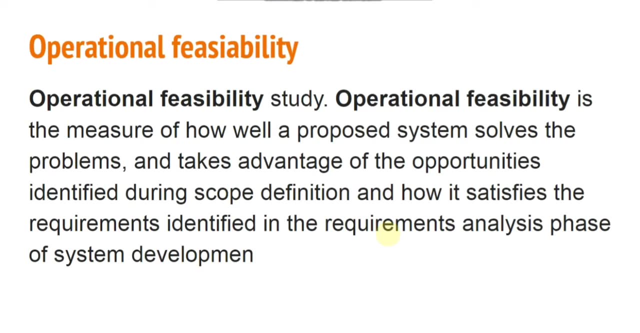 operation feasibility: schedule feasibility, economic feasibility and legal feasibility. So operation feasibility is the study of the mayor. How will the proposed system solves the problem? so operation feasibility contain the different Operation performed by the software and how the user problem will be solved. so it contains the operational. 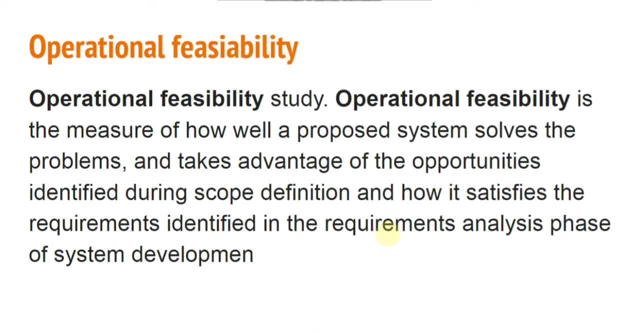 aspects of system and The task, advantages, opportunities identified during scope definition and and how it satisfied the requirement Identify in the requirement analysis. so how the record user requirement are captured. so it's all about the operation feasibility. the operation feasibility contain the operations performed by the System and how this, how the user requirement, are captured. 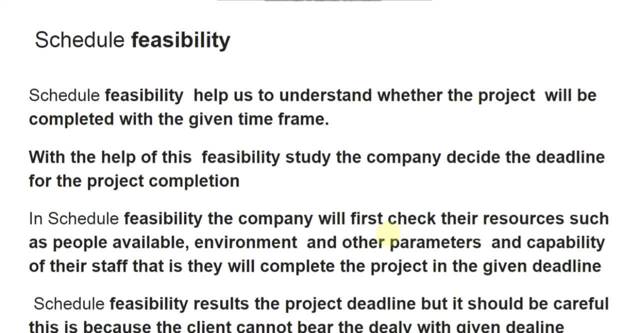 so Schedule feasibility. schedule feasibility mean time Time to complete the project. so schedule feasibility help us to understand whether the product will be completed with the given time frame. With the help of this feasibility study the company decide the deadline for the project completion. So in schedule feasibility the company will first check their resources, such as people available. 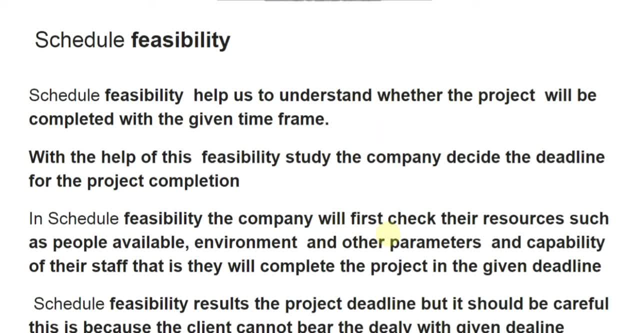 environment and other parameters and capability of their staff. their, That is, they complete the project in the given deadline or not. So schedule feasibility result: the project at line, but it should be careful. This is because the client cannot bear the delay with the given deadlines. So schedule feasibility help us to understand and help us to find that the project will be completed in the given. 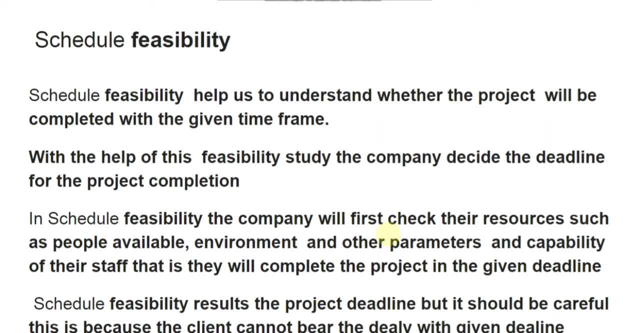 schedule are not, are we make extend the deadline of the software. so schedule feasibility very important from the perspective because if the company will fail to provide the project and the product to the user so it may lead a lot of loss to the company because the User want the software in the given schedule. 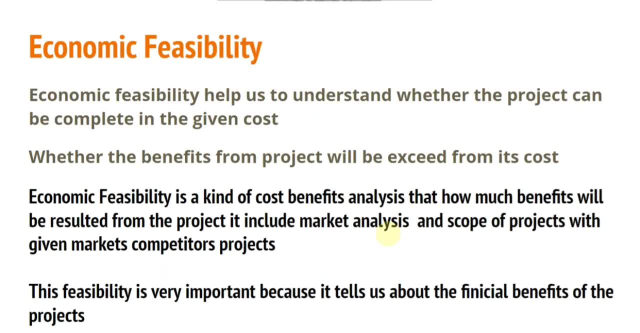 so economic feasibility. economic feasibility Help us to understand whether the product can be completed in the given cost or not, such as cost estimation, estimation, So whether the benefits from the project will be exceed from its cost. Economic feasibility is a kind of feasibility, is a kind of cost benefits analysis. that how much benefits? 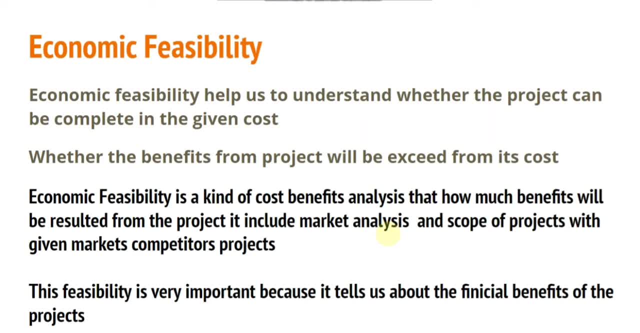 will be resulted from the project. It include market analysis and scope of projects with the given market competitors project. So this feasibility is very important because it tell us about the financial benefits of project. So economic feasibility is the study in which we estimate the cost of the project and we find out that how much benefits will take out the 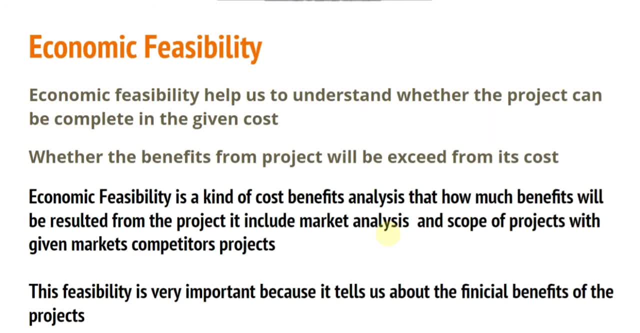 organization or the user from the given software product. So it is also a very, very important feasibility because it tell the both the user and the developers about the economic benefits of the project. So in economic feasibility we study the market analysis and the scope of project, whether the organization will get benefits from the software or not. so it both beneficial for